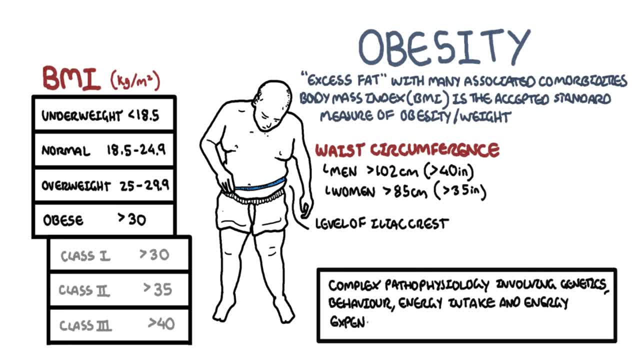 There is energy intake versus energy expenditure, as well as changes in the neuroendocrine pathways. But to put it simply, really obesity occurs when you have increased energy intake but reduced expenditure, And so all this accumulation of energy just goes into fat deposits around the body. 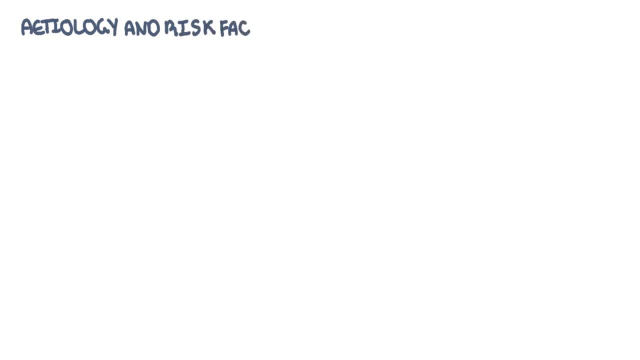 The etiologies and risk factors of obesity. it can be divided into behavioural things, such as physical inactivity. poor diet, such as high takeaway foods. also, cessation of smoking, because people take up other habits such as eating more. further, poor eating patterns. 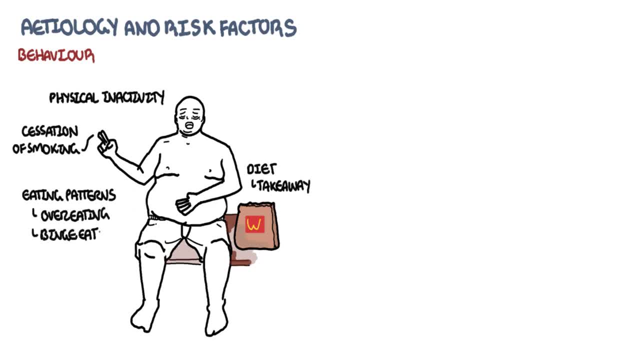 such as overeating, binge eating or night eating is associated with increased energy intake. Sleep deprivation- Sleep deprivation is also a risk factor. There are many medical causes of obesity. These include hypothalamic obesity caused by damage to the hypothalamus, a part of the. 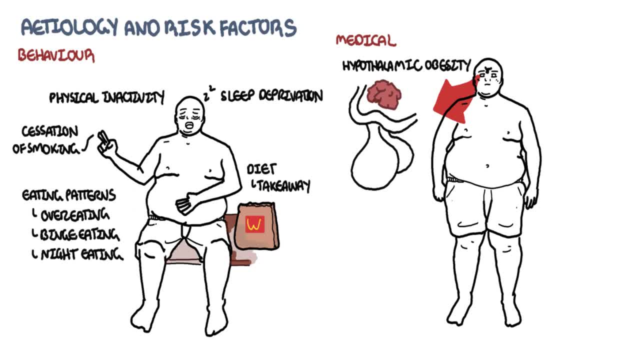 brain that makes hormones that control specific body functions such as sleep, as well as hunger, Growth hormone deficiency, hypothyroidism, low thyroid levels released from the thyroid gland, hypogonadism In women, polycystic ovarian syndrome. 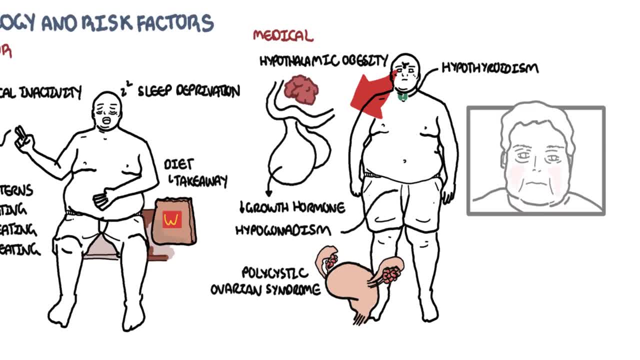 Which is also associated with hirsutism. Cushing syndrome is a very important medical cause and really patients manifest with elevated cortisol levels and you could get moon like faces and a buffalo hump. There are many medications that can cause increase in weight. 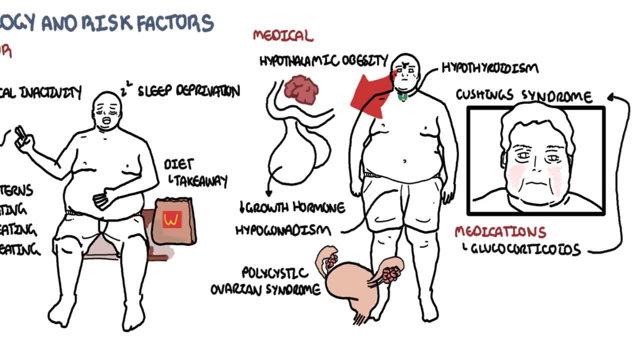 These include namely: corticosteroids, which really lead to Cushing's appearance and stimulates appetite, so you eat more. Antipsychotics, Antidepressants, Beta blockers. There are also anti-diabetic agents, such as insulin, which causes mild weight gain as 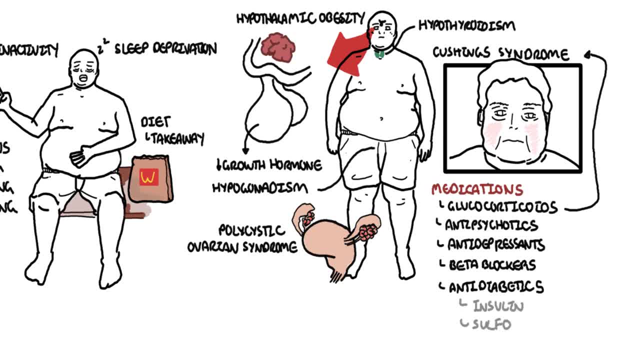 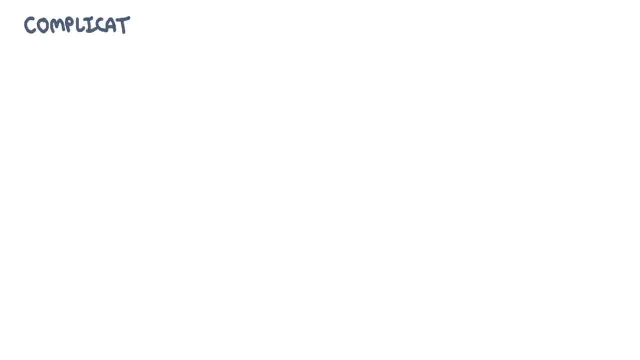 well as sulfonylureas. Complications of obesity include stroke, the stigma associated with being obese, respiratory issues such as obstructive sleep apnea, Hypoventilation syndrome, which is really characterized when you have slightly increased amounts of carbon dioxide in the body. 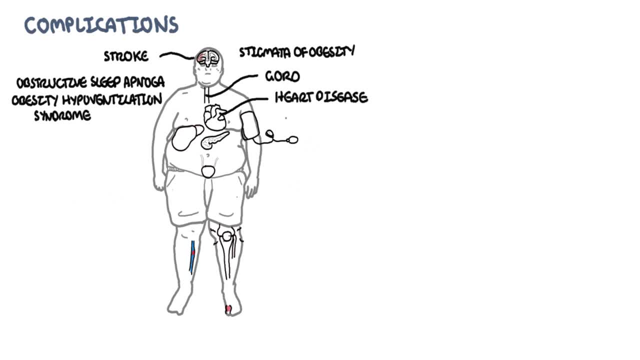 Gastroesophageal reflux disease, Heart diseases, including heart attacks, hypertension, hyperlipidemia, a fatty liver disease, diabetes, urinary incontinence, osteoarthritis from all the weight, Increased risk of gout, venous thrombosis, hernias, as well as a increased risk of certain 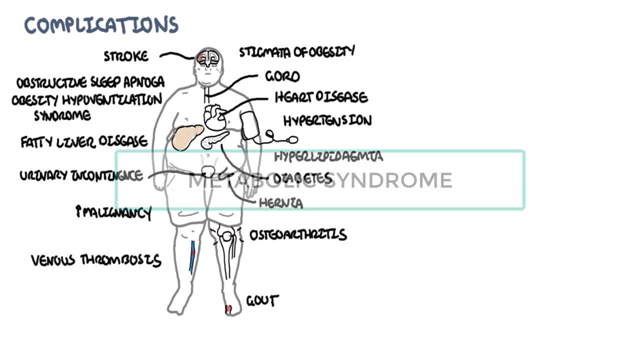 malignancies as well. Important to know something called metabolic syndrome, which is really encompasses obesity as well. Metabolic syndrome describes a constellation of medical condition which increases the risk of cardiovascular disease. These conditions include insulin resistance, Hypertension, Hyperlipidemia. 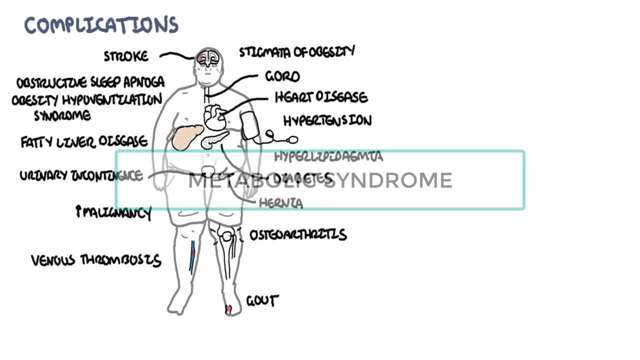 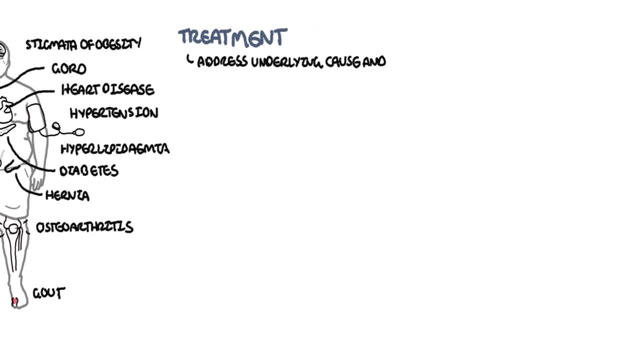 Obesity. All these make up metabolic syndrome. The treatments for obesity: Well, there are many approaches, but first is to address the underlying cause, if it's medical or behavioral, as well as addressing the triggers. You want to set a realistic goal, for example, 5% body weight reduction per year and good. 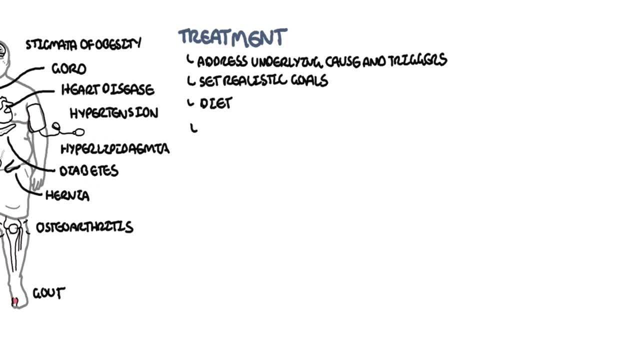 idea to create an action plan involving a certain diet, Such as a low-fat diet Or a low-fat diet Or a low-calorie diet, An exercise program, Pharmacotherapy or medications also have a role in the treatment of obesity, usually when all other things fail. 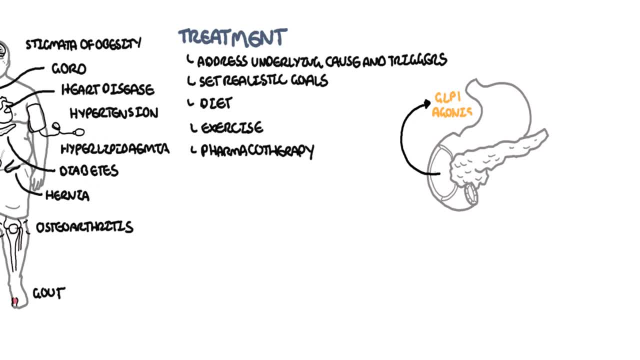 These pharmacotherapies include a GLP-1 agonist. Now, a GLP-1 is a normal peptide that's produced by the body, which slows gastric emptying, inhibits glucagon excretion and stimulates insulin production. The side effects of this include nausea and vomiting. 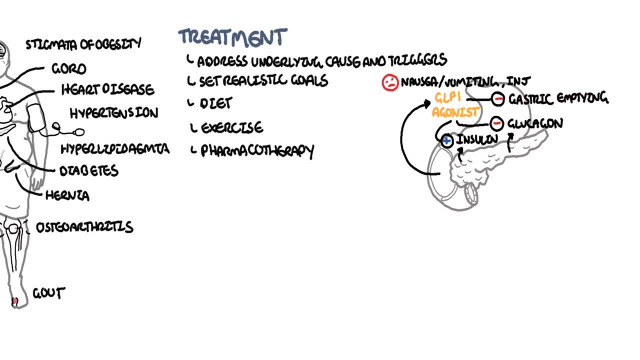 Further, GLP-1 agonists are given as an injection into the tummy or the thigh, and so this could also be a side effect in a way. Orlistat is another medication that works on the pancreas by inhibiting the pancreatic. 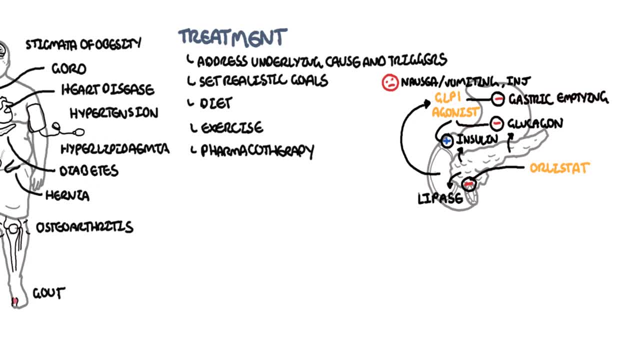 lipase. Lipase is an enzyme which helps break down fat so that fat can be absorbed by the body. By inhibiting fat absorption, you're essentially breaking down fat. By inhibiting fat absorption, you're essentially breaking down fat. By inhibiting fat absorption, you're essentially breaking down fat.